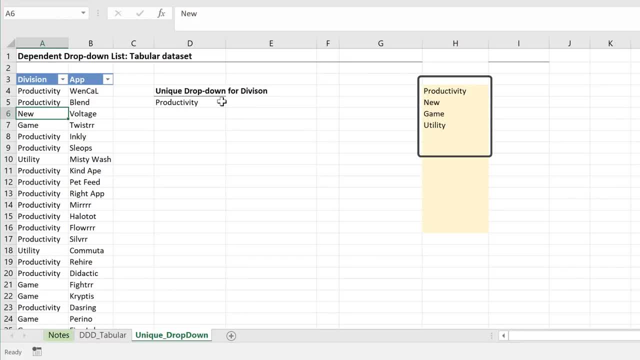 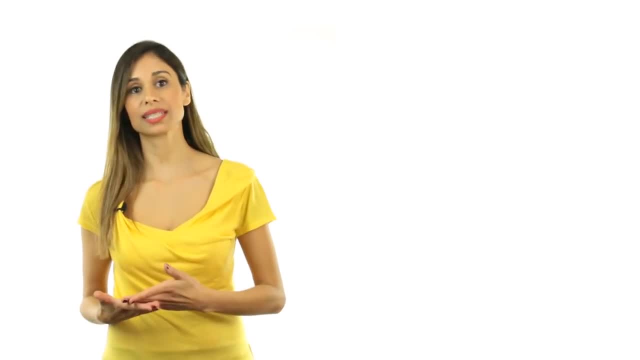 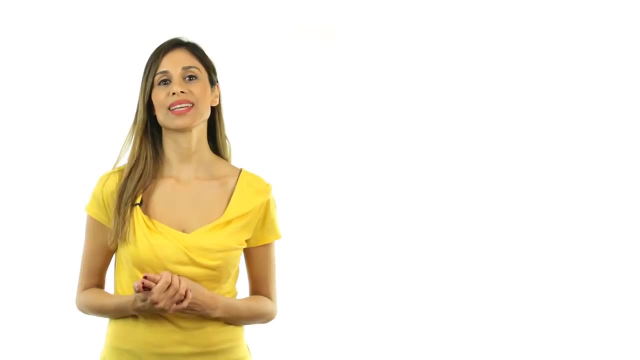 Here's how it looked. I'm also going to add the link to that video in the descriptions. We also used Excel's table feature to be able to add more names and have them reflected on our dropdown list. Then the next question came on: how could we create the second dropdown? 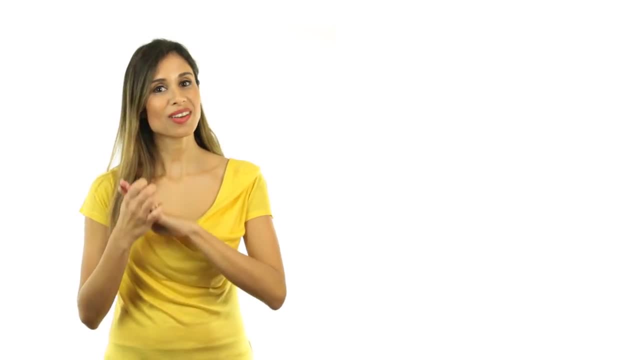 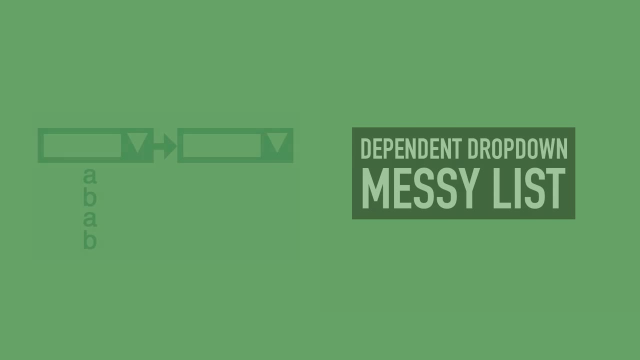 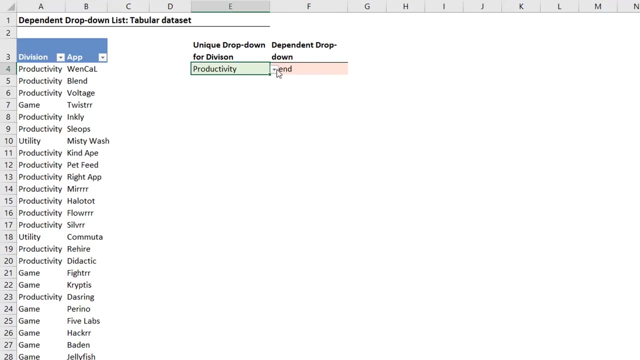 that's dependent on the first dropdown and based on the same messy data set. So, for example, if you select productivity from this list, we want to see all the apps that belong to productivity. If you select games, you want to see all the apps for games. 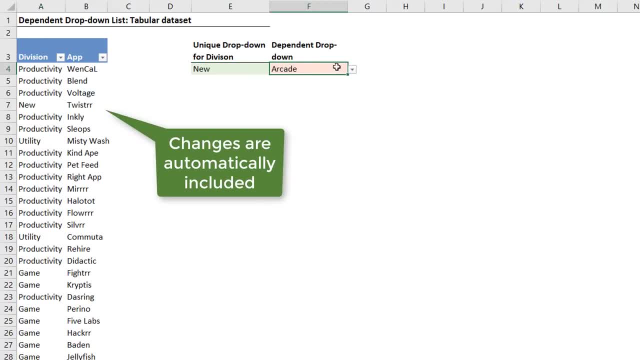 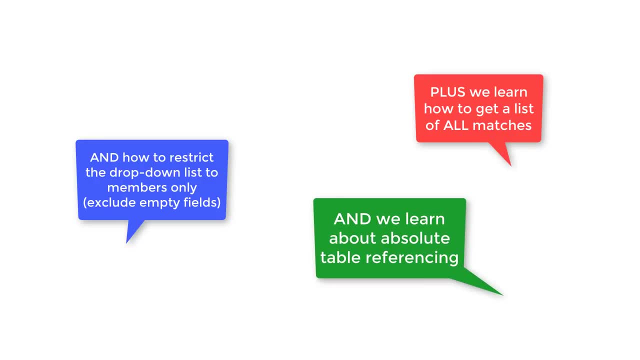 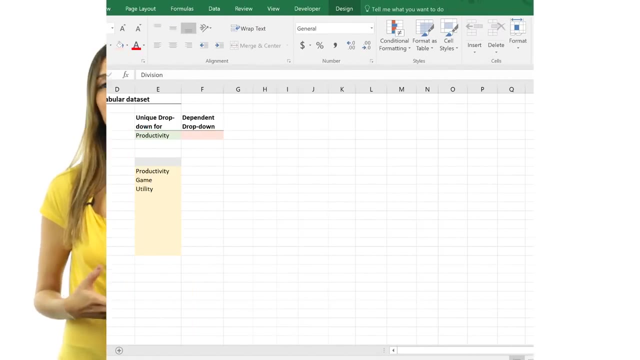 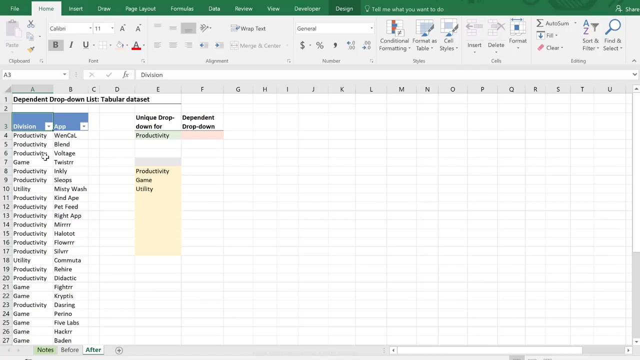 and so on. So let's see how we can set this up with a formula that doesn't require control, shift, enter. Let's just take a look at the data set that we have. Division is listed here. It's random. They're not grouped together. 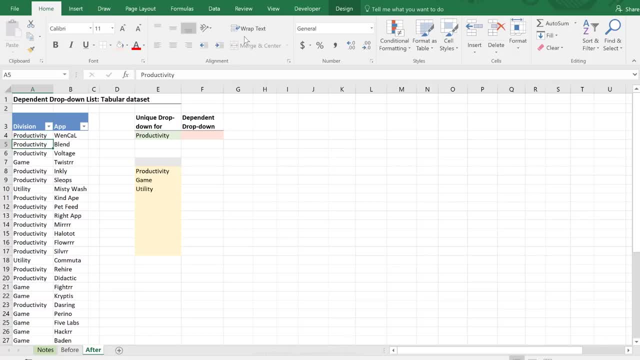 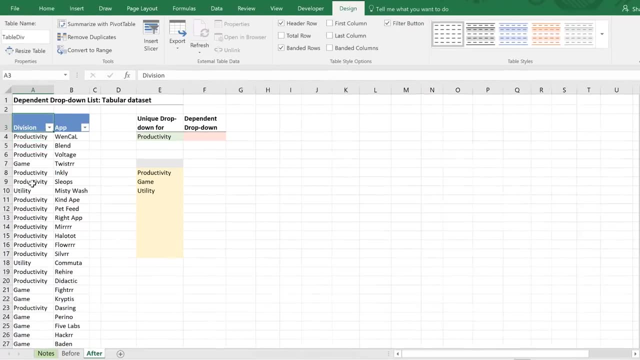 We have the apps listed in front of the division. I've created a table out of this, called table div. In a previous tutorial we sought for getting a unique list out of the division, So in this case we just have three divisions here. 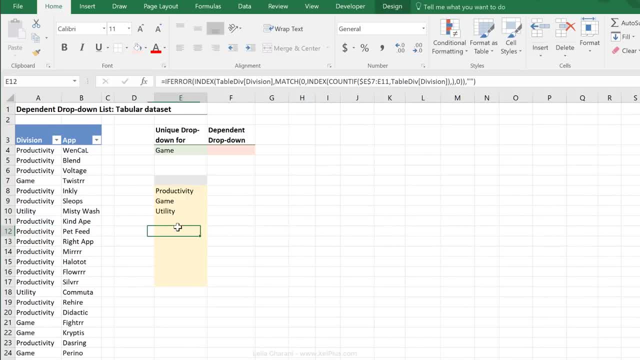 If we got new divisions added to this list, our data preparation table, which was actually the driver for this dropdown, would update automatically. As a result, our dropdown updated automatically because behind this there's the offset function. Now, if you missed that, 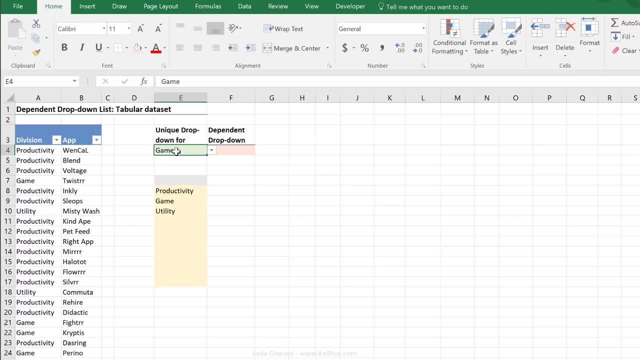 the link to it is in the descriptions. But in addition to this, I really recommend that you watch the video from Kevin Larbas, where he included many different ways of getting the same thing done. So if you have a huge data set and this formula approach could be a bit slow for you. 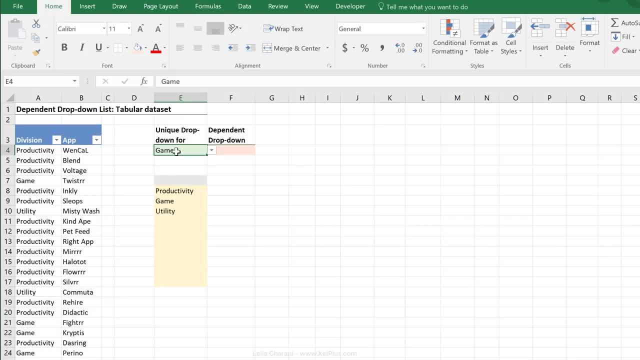 I do recommend that you check out your other options from that video And I'm going to add the link to that as well in the descriptions. This video is for those people who are interested to see how you can get the dependent dropdown. This is the dependent dropdown part, also with formulas. 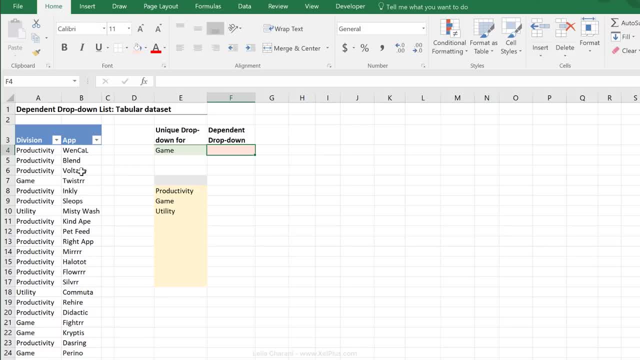 Okay. so right here we're going to have the apps that belong to the game utility, And if we switch to productivity, we're going to have the apps that belong to productivity. So my approach here is very similar to what we did to solve for this one. 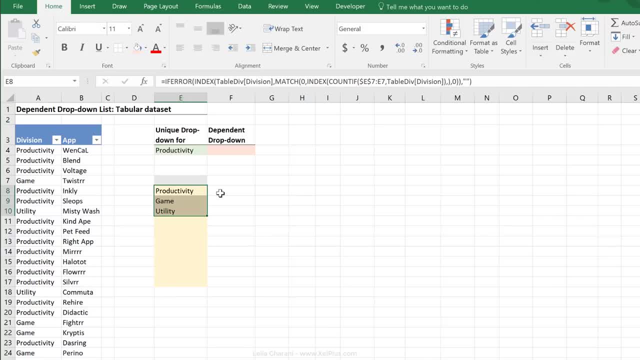 I'm also going to use a data preparation table and get the list of apps in the data preparation table and then make a dropdown based on that, This data preparation table. we'll look slightly different because it's going to be going this way instead of vertical right. 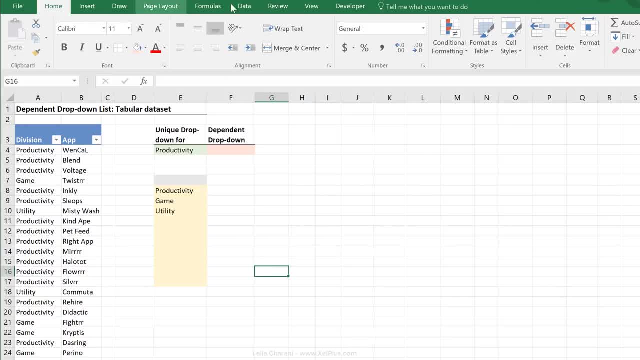 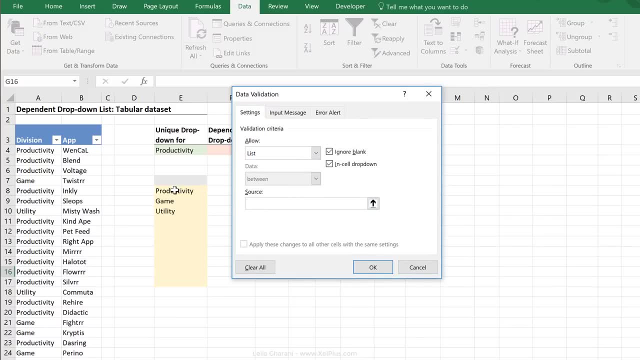 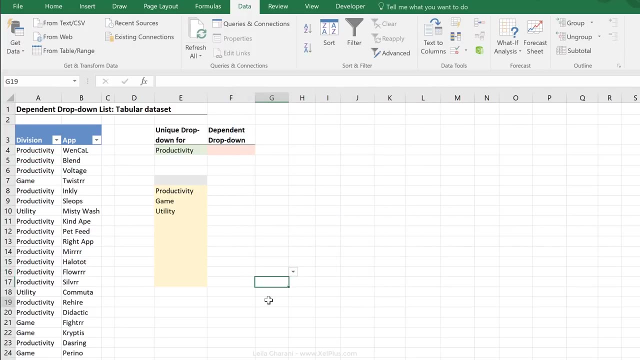 But that doesn't pose any problems for the data validation right. If we go to data data validation and we select list, it doesn't matter if our list is vertical or horizontal, it's still going to show it to us in a vertical manner, right? 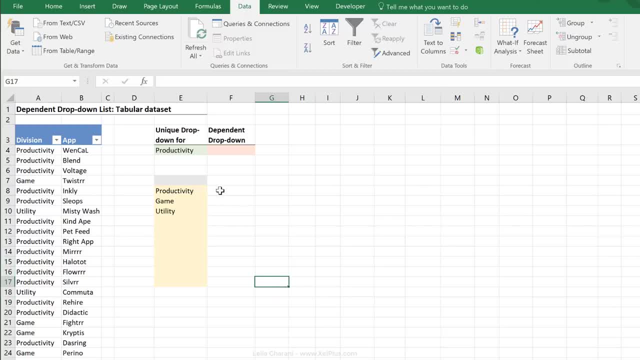 So if we manage to put our list in a horizontal way in front of the table, we can see that it's going to show us that we've solved the problem. So if we go to the table, we can see that we've solved the problem. 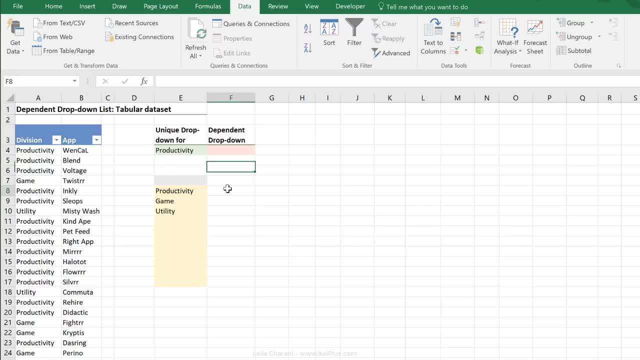 And then we can also use a similar function like offset to get the correct list shown. then we've solved this problem. Next challenge to solve for is the formula that we need for this, And I mentioned that I want to use a CSE-free version. 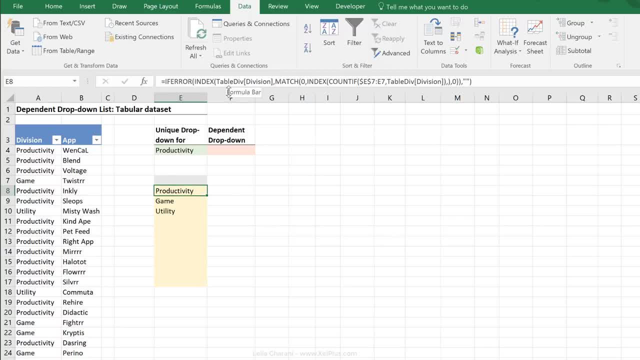 of a formula. So this means I have a choice between index, which is going to work well with getting the answer from the app column. I'm also going to use index in here, right? Because if I manage to find the row that the apps are sitting on based on the division here. 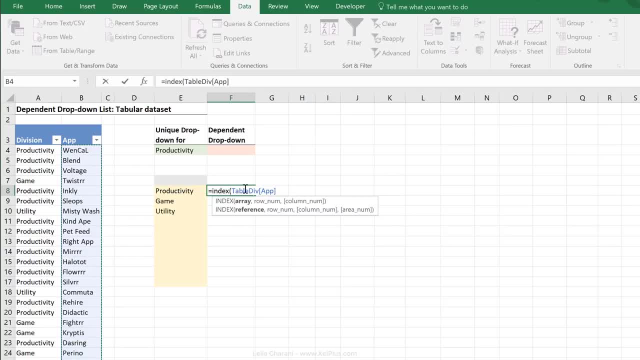 then I'm all set. Remember what the index function needs is first is the map and then how many rows it should go down, right. So if it checks that this is productivity and it notices, okay, the first occurrence here is in position one, then I have my answer. 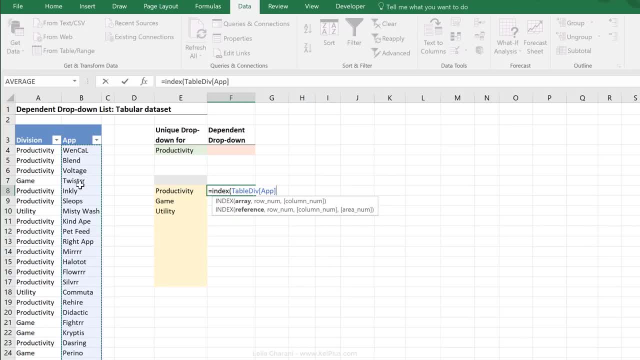 Second occurrence, position two. third, position three, and then it needs to skip position four, because the next occurrence is actually in position five, Right? so the challenge for the index function here is to find the correct row number. I'm just going to put the rows that we would need. 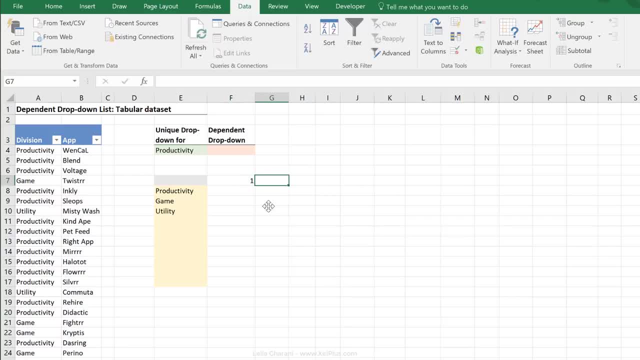 for productivity, for example, in here, just so that we can double check our formulas later. so that would be: one, two, three and four is not a match right, Because one, two, three is a match. This one is game right. 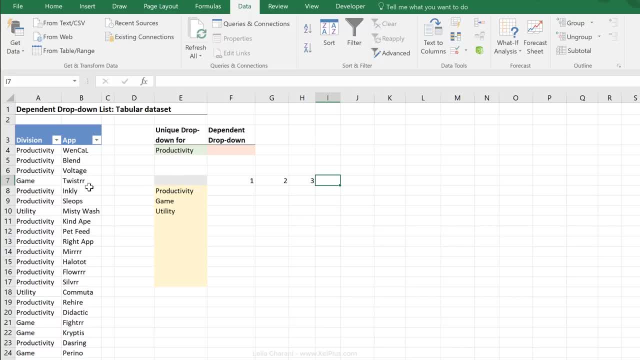 So for productivity, this will not be a match. Then we need five, and then we need six, and seven is not a match and then we need eight. Okay, so something like this is a sample data set that we can compare to when we manage to come up. 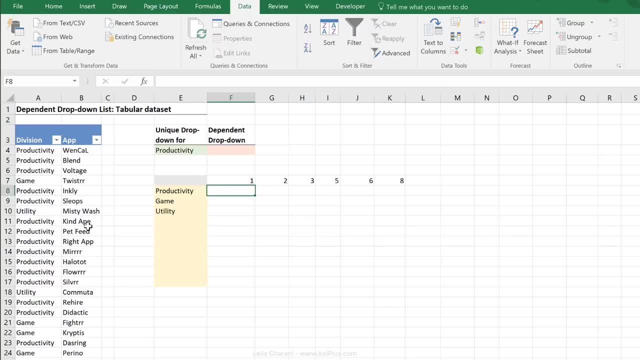 with a formula that gives us these numbers. So what formula could we use that is also CSE-free? I can think of the aggregate function, because inside aggregate you have this part here that can handle arrays. I would probably go with small to get the apps shown. 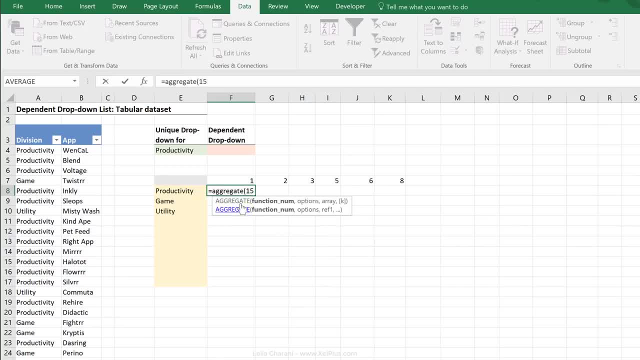 in the same order that I see here right, And the good thing with the aggregate function is that you get this additional options of ignoring error values, and that's something that could come in handy When we also select small and we put in our array. 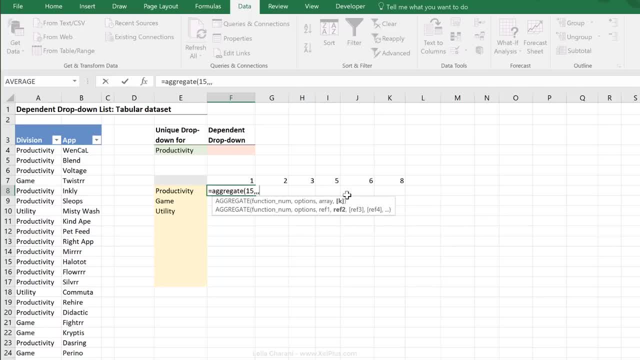 we get this additional option of ignoring error values, and that's something that could come in handy When we also select small and we put in our array. the last argument is, if we want the smallest, the second smallest, third smallest and so on. 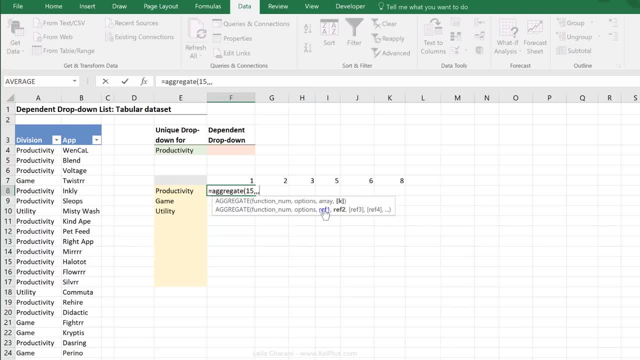 and that's something that we can also make dynamic. But even if we have an idea about the formula that could work, the challenge is to get this array part right that is going to give us these numbers inside the array. Okay, so let's start with the core first. 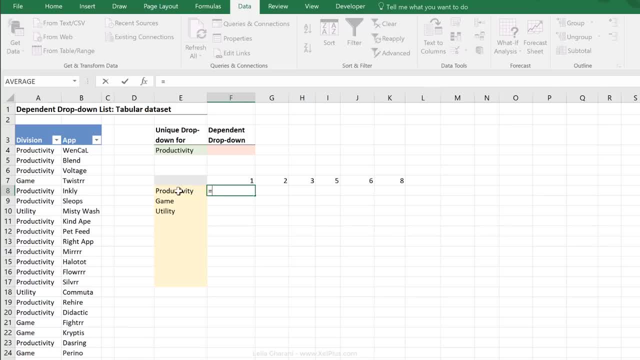 Let's look at how this array could look. I need to check If division- okay, and I'm just going to click on top to get the whole column of the table. if division equals this, Okay, I'm just going to press enter. 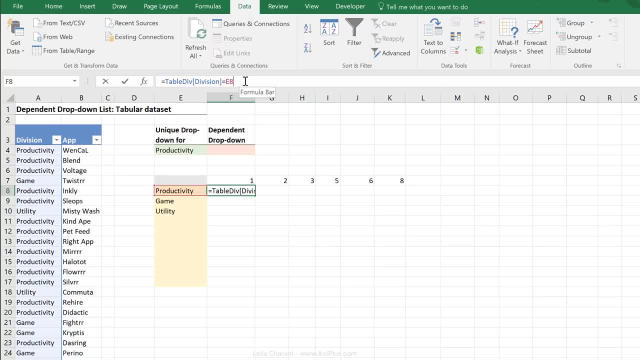 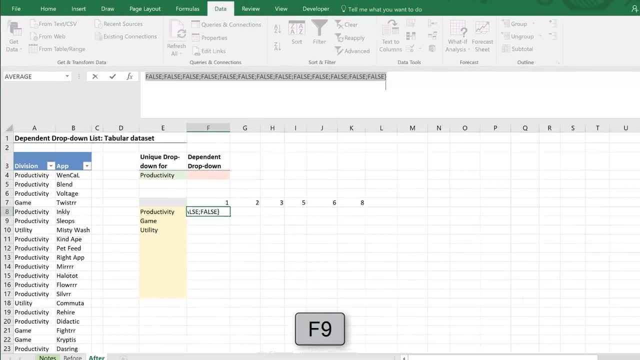 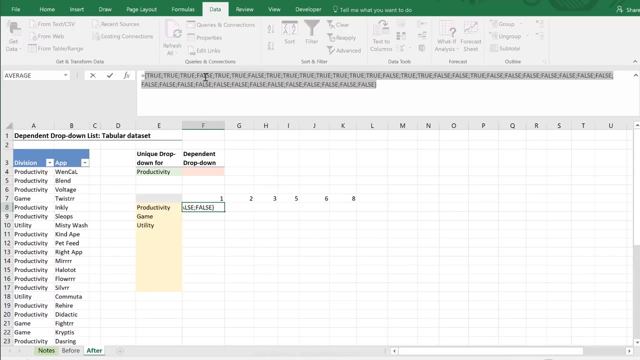 Now this is an array formula all written in one cell. To see what's really behind it, we need to click in the formula bar and click on F9.. Let me just expand this so we can see the whole data set. We see that, for the first occurrence is true, true, true. 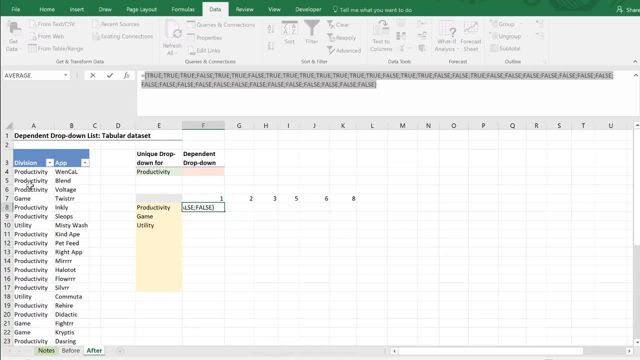 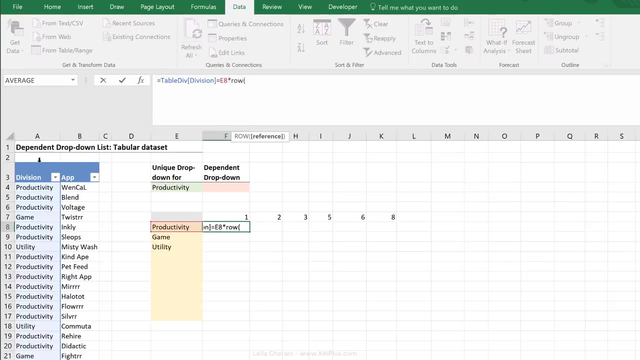 false, true, right. So that's exactly what we see here. Now it would be great to translate these to row numbers, So I'm going to press Control Z to go back to my formula and multiply this with the row that they're sitting on. 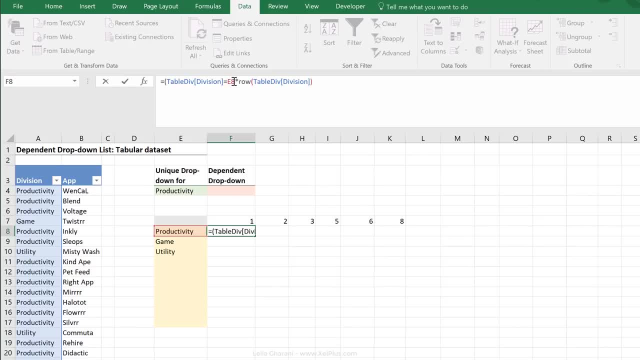 Okay, but I'm just going to put this in brackets. And now let's press F9.. We see now the associated row number of productivity. right, So four, five, six, then it's zero, because there's no match there. 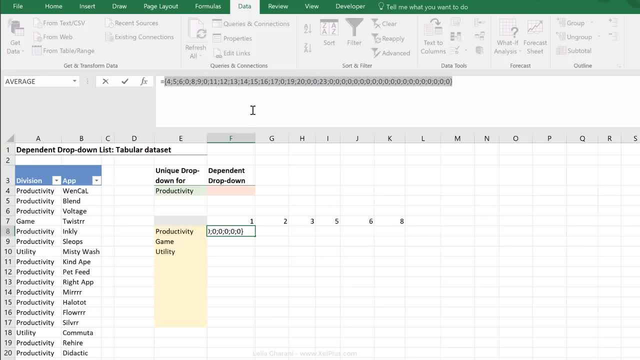 eight, nine, zero and so on. That's good, but if we're planning to use small on this data set, then small is going to always find all the zeros right. We want to get rid of the zeros, and best would be, since aggregate can ignore errors. 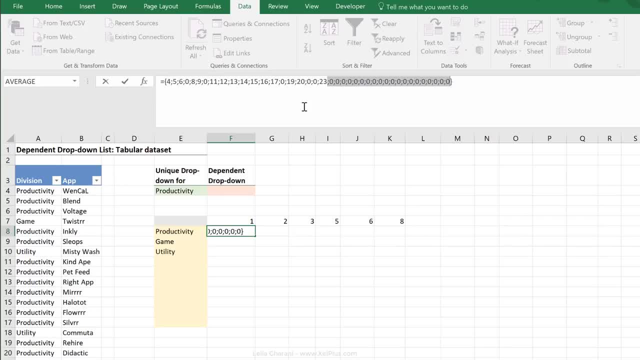 that we actually generate an error wherever we have zeros To do that. we can divide this, which is the result of our true and false values, with itself and then multiply it with the row. Why? Because if we divide a true with a true, 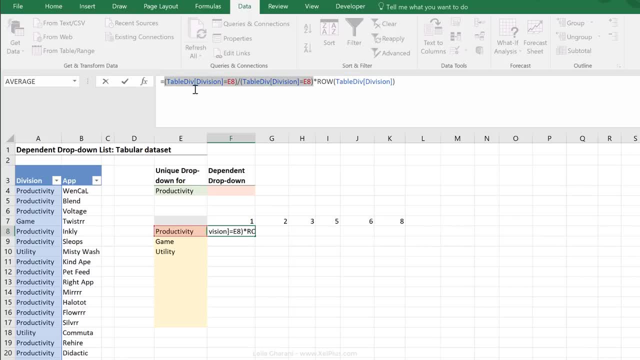 we're dividing a one with a one, we get one. If we divide a false with a false, we're going to get an error, because we're dividing zero with a zero right. So if I just highlight this and press F9,. 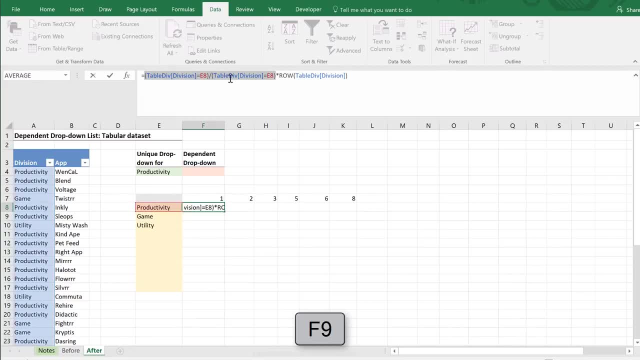 you can see one one error, one one, and so on. Now, if we multiply this with the row, we should get the same thing, but have the zeros replaced with errors. Okay, so we're on a good track. 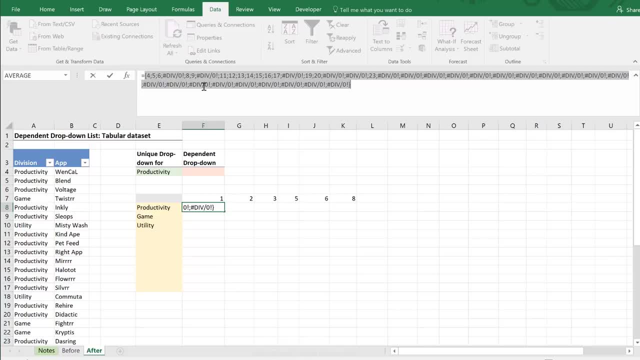 Since we're planning to feed these later on to the index function and if you're indexing this area, we need to start with one, two, three and so on- we need to make a correction to these numbers so that they also start from one here. 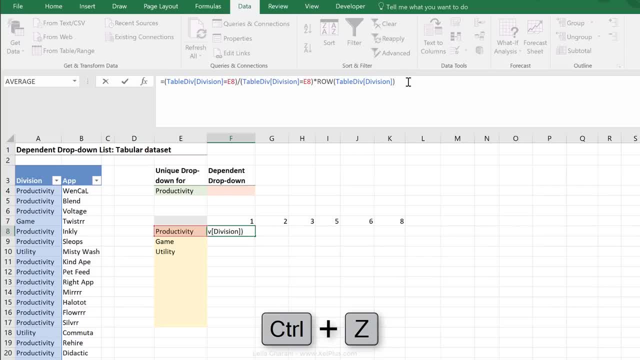 Okay, so I'm just going to press Control Z to go back and I need to deduct the header row, So I'm just going to click on this one right here, close bracket, and since we want this result to be then multiplied with this one, 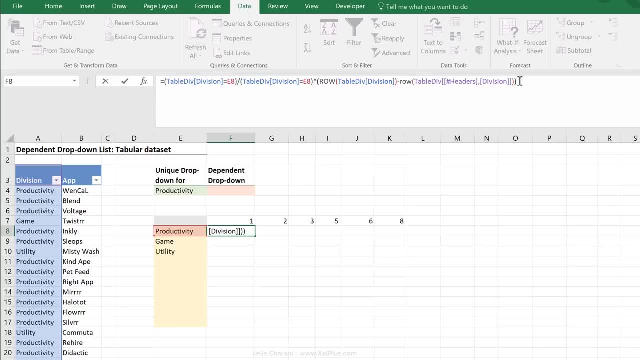 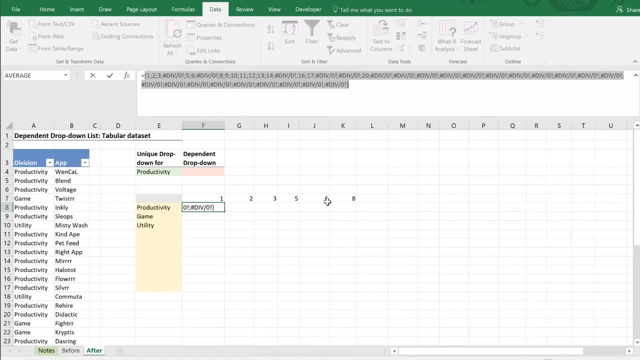 I have to put the whole thing in its own brackets. Okay, so now let's check. One, two, three, error Five, six. very good, then it's eight. Now we're on the right track. We can plug this in the aggregate function. 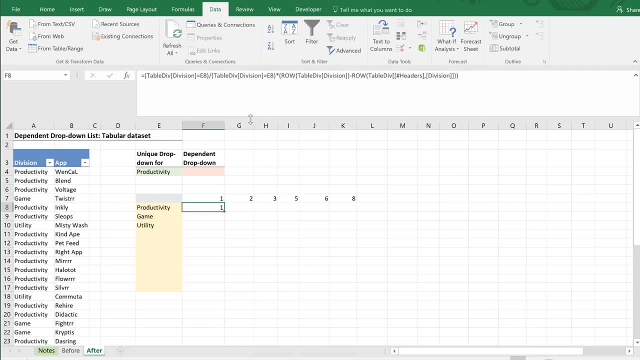 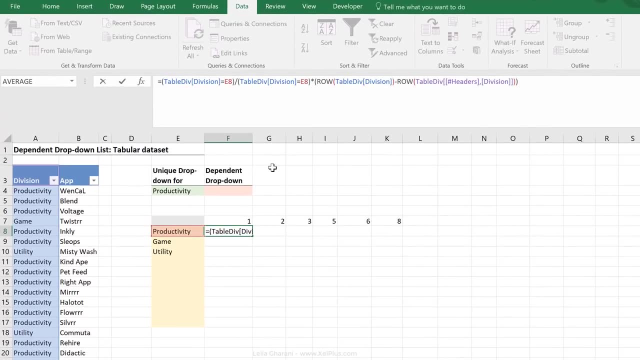 We can plug this in the aggregate function. We can plug this in the aggregate function, But let's just think about the fixing as well, because I'm planning to pull this across and pull it down as well. So I don't want this E8 to move. 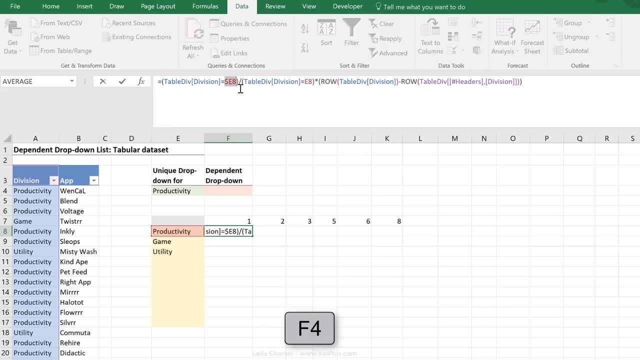 so I'm going to fix that, but I do want it to move down right, So I just need the column to be fixed here as well. The rest are table references, so let's see how they behave later on when we pull this across and down. 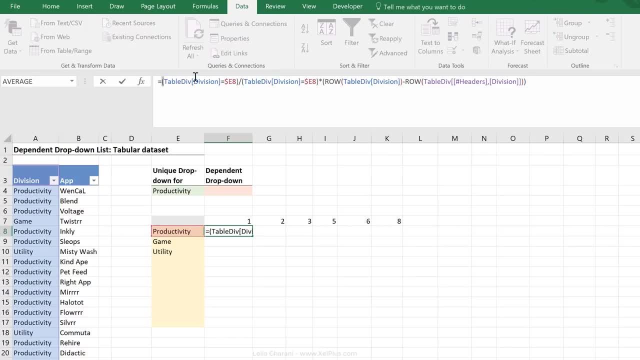 Let's plug this in our aggregate function as the array part. We're going to go with number 15, which is for small. Then we're going to ignore errors. Now you can also pick six or pick three, which ignores also hidden rows. 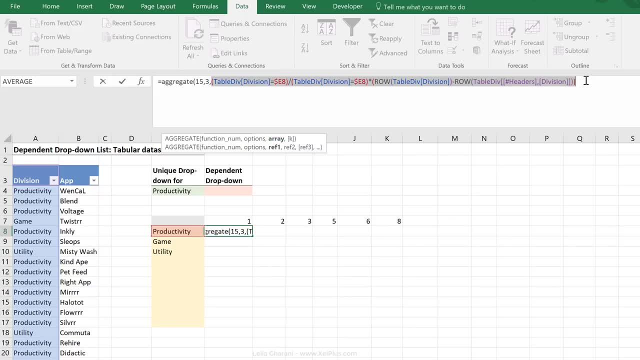 Then we want our array, which is this. Then, after this, we want our K. So if it wants the one small, then we want the K. So if it wants the one small, then we want the K. 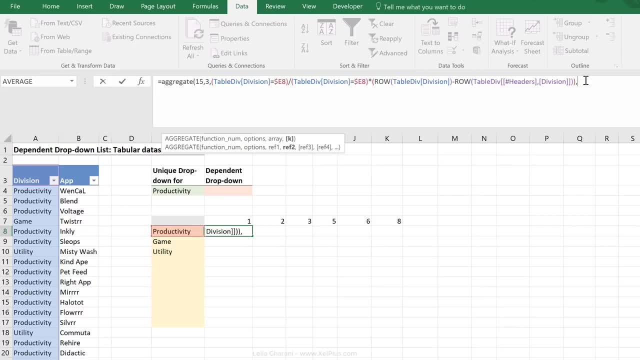 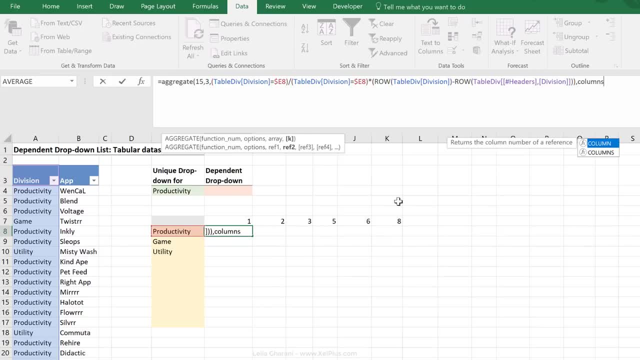 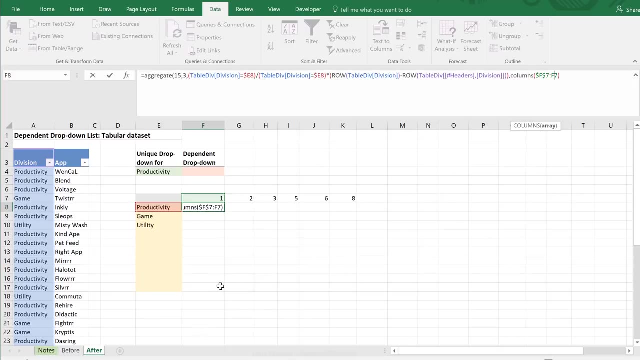 when we're dragging this across. So here we can use the columns function and just take a look at the column above and fix the first cell reference. The second one I can leave as is, but if I don't want it to come down, 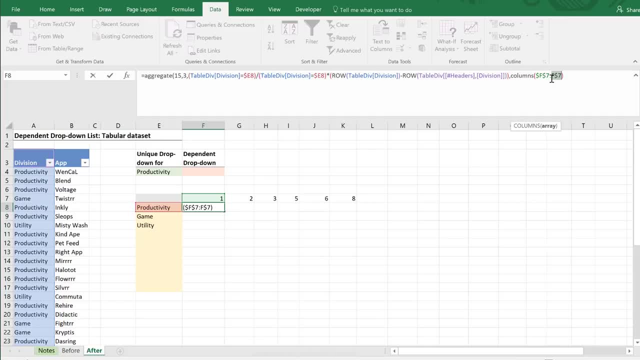 I can also just fix the seven and leave the column column variable, But that doesn't matter. you can also leave it fully variable. That should take care of the aggregate. Let's just check what happens if we pull this across. So this looks good, this looks good, these don't look so good. So what's happening here? 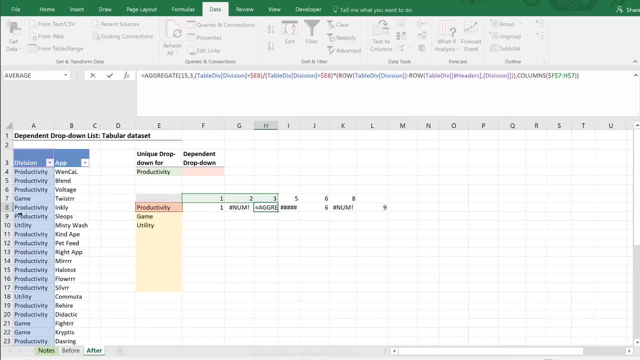 It shifted to the app. What's happening here? It shifted back, So tables behave in this way that when you're pulling it across, your column reference is also going to move, and then, when the table ends because it can't move anymore, it's going to go back, But we 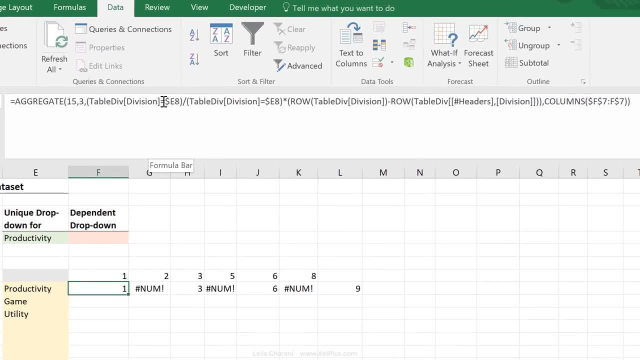 don't want that. we want to fix the column reference to division. And fixing in tables means that you need to get that square bracket header part and do a column and then reference it again. So it's like division to division Kind of like when you're referencing a column. 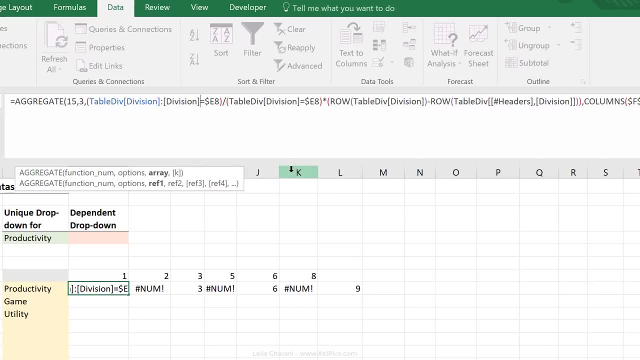 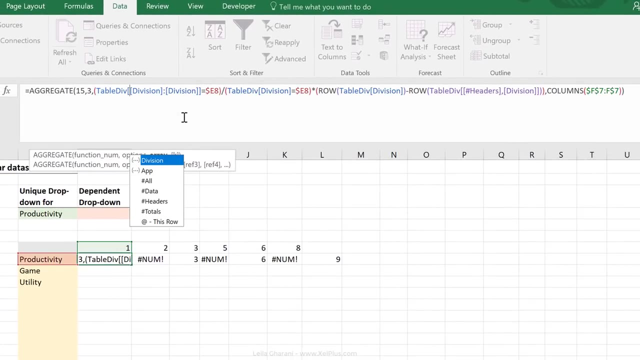 as an entire column, Like for this one, it would be K to K. It's the same, except that you can't leave the formula like this because there is an error in here. it doesn't accept it. You need to put them in square brackets again. So that whole reference in square brackets. 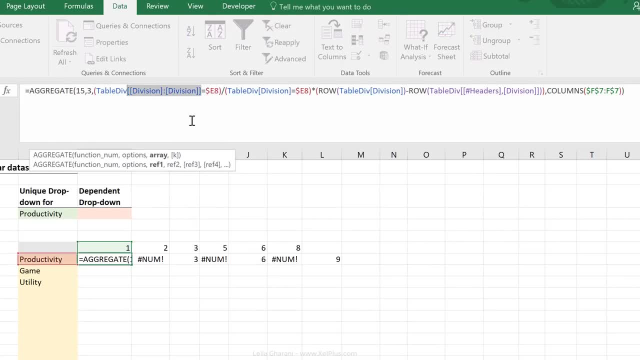 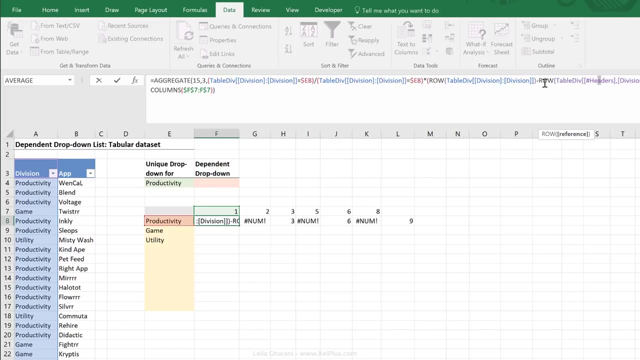 So now I can leave it. The main challenge here is to find your square brackets on the keyboard. I'm just going to update All of these ones that need the fixed referencing For the header, since I'm only interested in the row number. if the header switches to here and back, it doesn't matter. 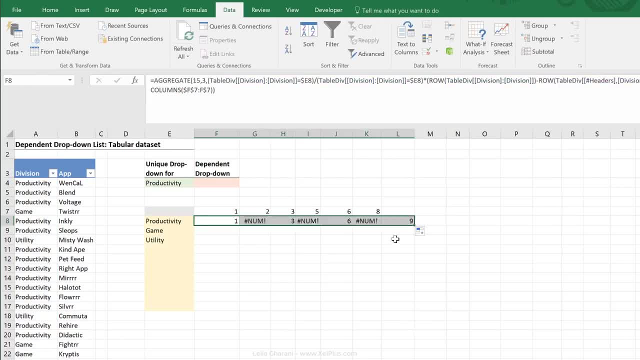 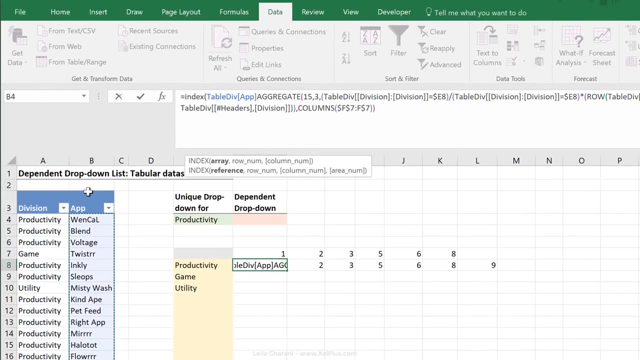 I can let that switch Now. if you pull this, it looks good. It's exactly the numbers that we want. So now we should be able to plug this inside an index function. We need to index app here, because our answer is an app. But again, we don't want it to end up in space. So that's where we're going to set up the index function. We need to index app here, because our answer is an app, But again we don't. I don't want it to move back and forth. 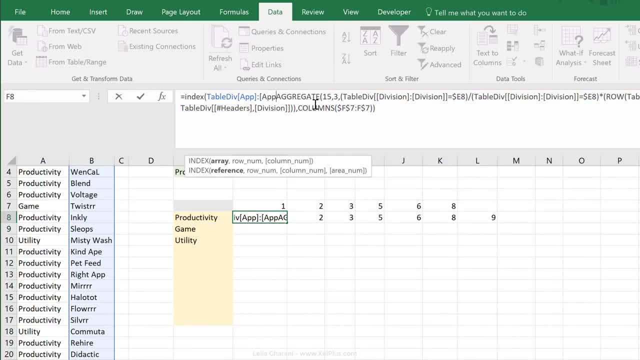 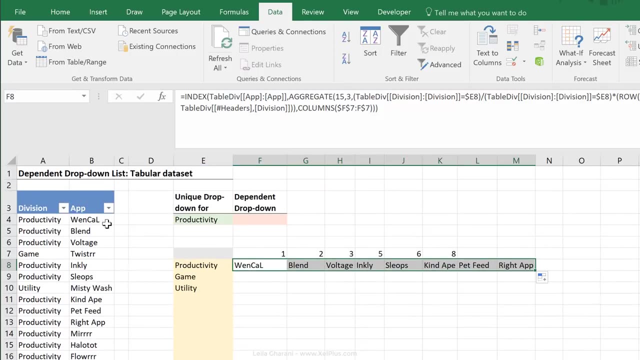 so we need to make sure that we have a fixed header here and do this special referencing with the square brackets And that's it, and let's close the bracket there and see what we get. Okay, let's just check these. Wenka Blend Voltage, Twister, Skipped Inky. 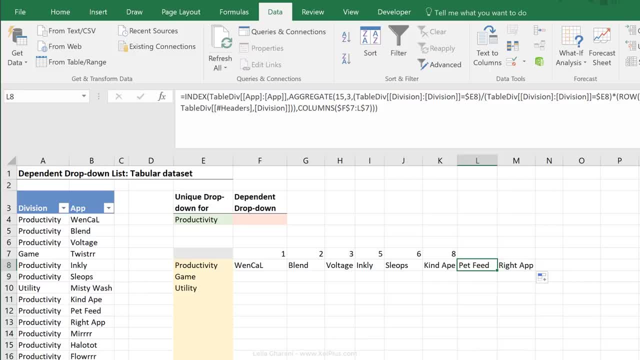 Sleops, Kind Abe and so on. Okay, so that looks really nice, But now the thing is that if we add more productivity apps to this, we want our formula to pick it up. So we do want to leave enough space here. 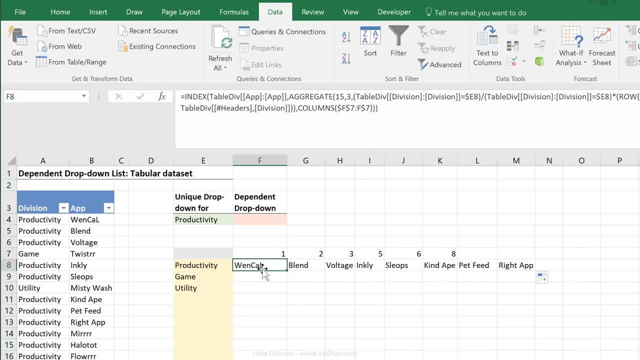 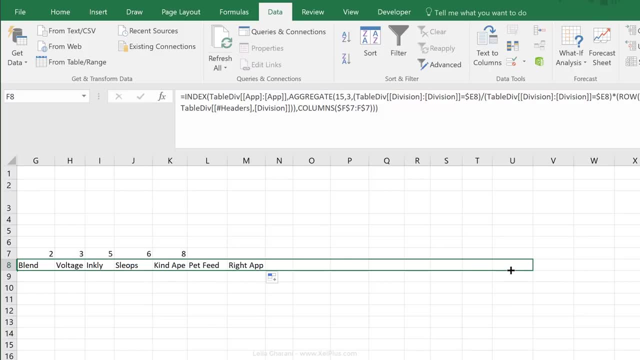 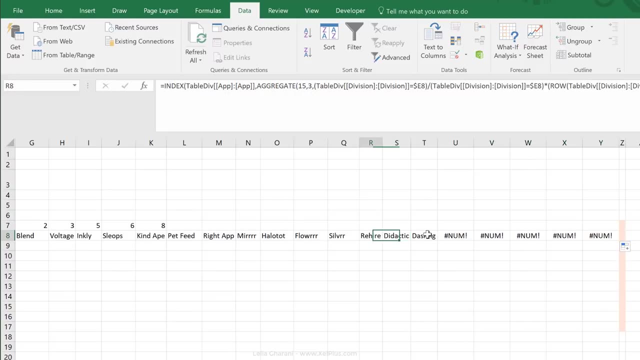 just like we left enough space here to account for new divisions. So I'm going to pull this across until where I think I might have apps being added. Okay, so I'm going to go until here And we get errors wherever it doesn't find anything. 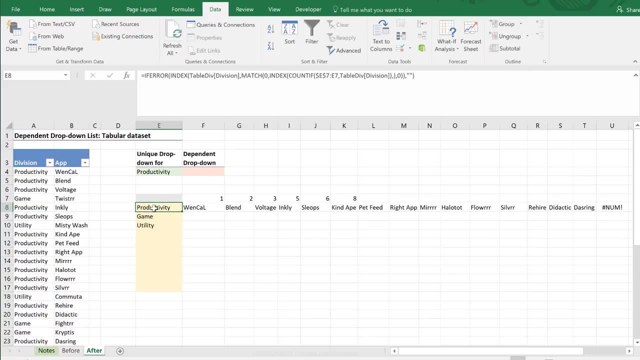 and we can correct for these errors. instead of using if error, let's do a count. We can count how many productivities we have on this list and we'll make sure that the moment our columns are more than this count, we're just going to write nothing to the cell. 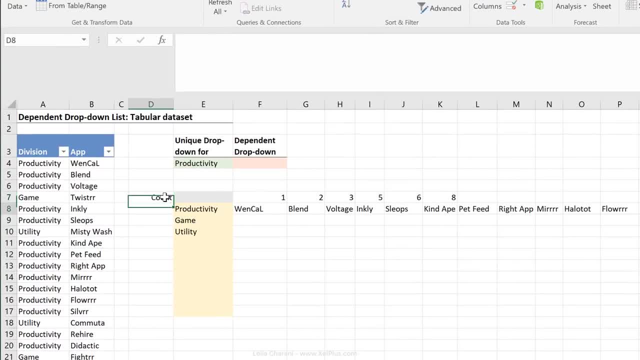 instead of the error, Let's just use this helper cell here and do a count. if our range is division and our app is this one, Okay, so I'm just going to pull this down. That's the count. So let's add our if to this. 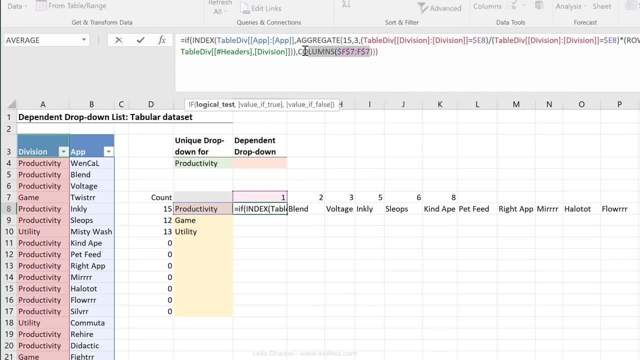 If the columns- here we can just copy this formula- is less than or equal to our number. here And again, let's think about the fixing. We have to just fix the column but not the row. Then it should do the index thing. 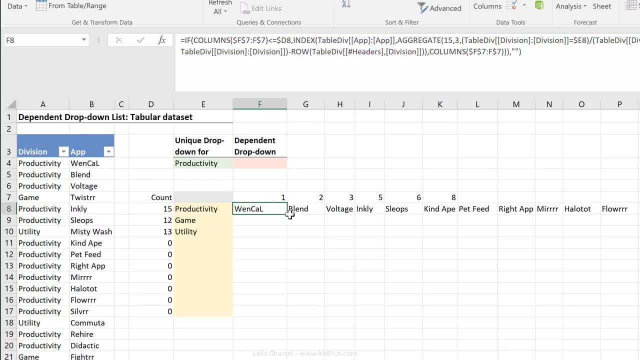 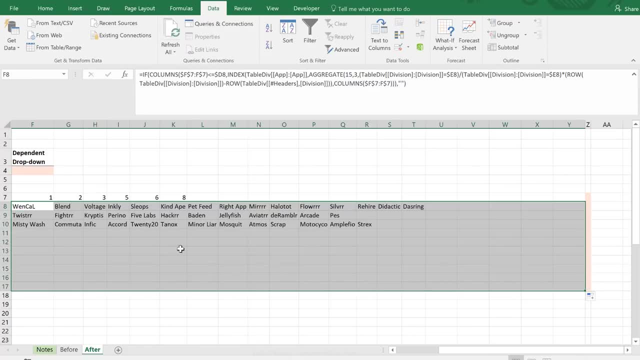 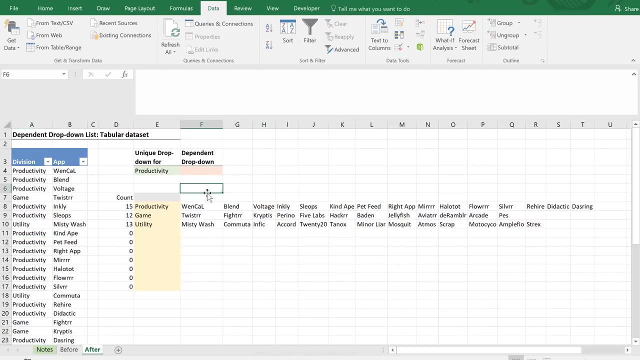 Otherwise it should do nothing. Now let's check. Looks good, And the real challenge is to make sure everything else updates as well. These look good as well, So I can get rid of this helper one Now that I have my app list here. 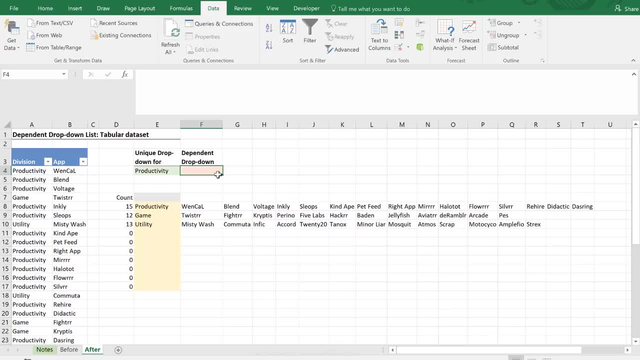 I just need to create a dependent dropdown Here. I will also use the offset function, just like I did here, except for this one, Except that it's going to have a bit of a twist to it. We need to figure out which row our list is sitting on. 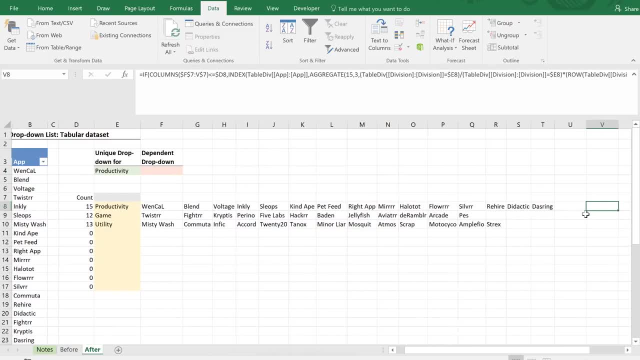 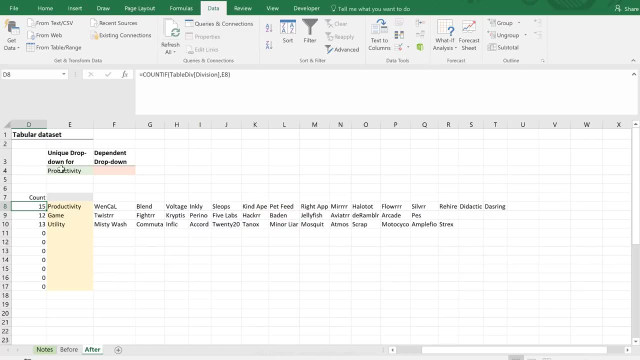 and how many columns our row has. We can fix the columns to 20,, for example, in this one, but we'll just see the last ones, the last places as empty on our list, And you'd probably want to restrict that to just the number of apps that you have on the list. 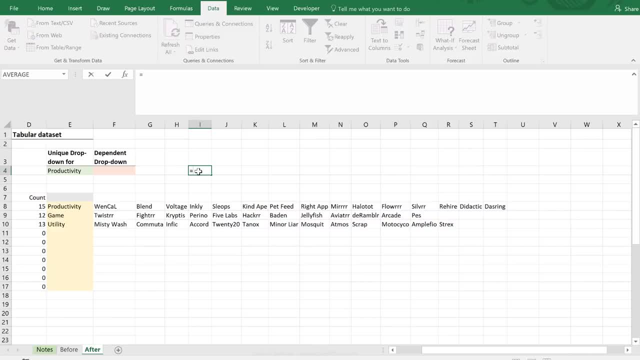 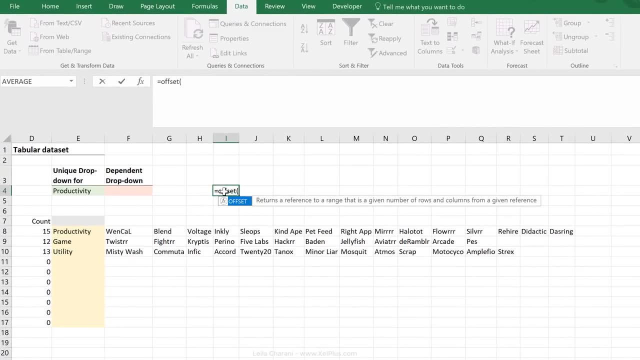 Right. So let's see how we can overcome these challenges. I'm going to type the formula for the validation list in here first, and then we can copy it to the validation. It's just easier to track. So, offset, our starting cell can be this one: 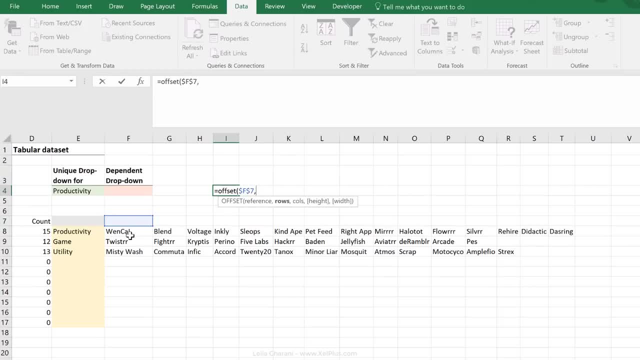 I'm going to fix it. Then, how many rows do we want to move down? So which list do we need? Well, that depends on our first selection, right? So I can match for this one, and I'm going to fix it in this list. 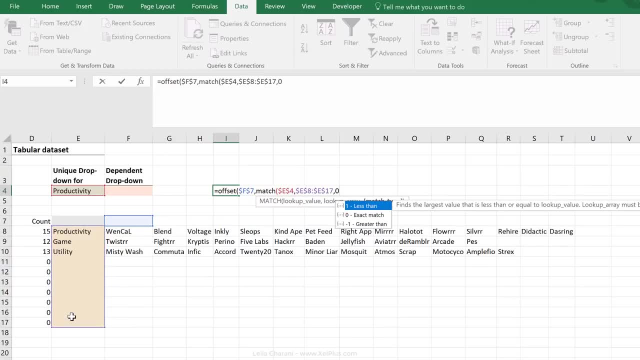 Fix it again and I want a perfect match. And for the columns, how many columns do we want to move? Well, we don't want to move any columns, We want to include all the columns. Including all the columns is the width argument of offset. 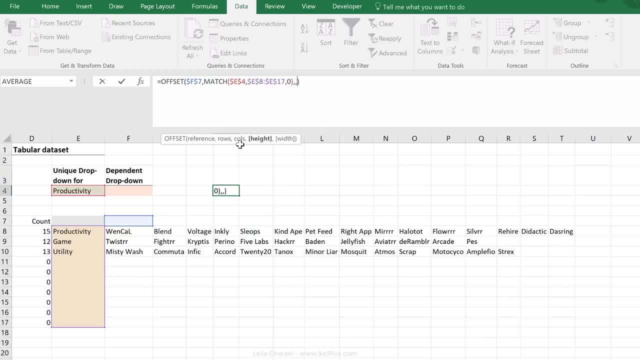 For the column argument. since we don't want to move anything, we can skip it. Height is one that's an optional argument. we can skip it. Width is how many columns do we want included. So the easiest approach is to accept those empty ones. 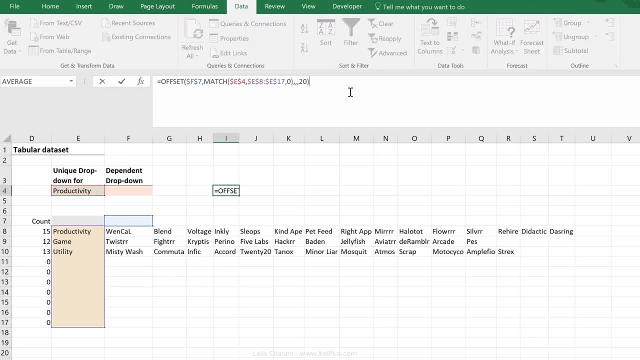 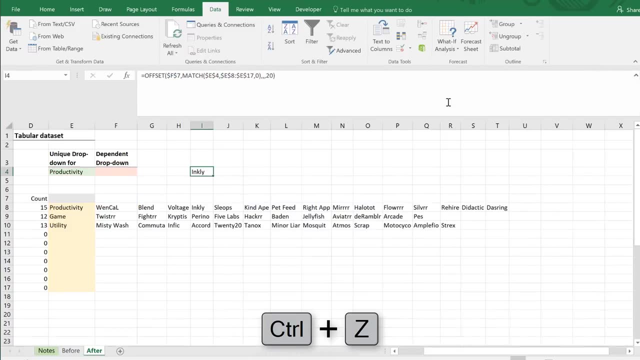 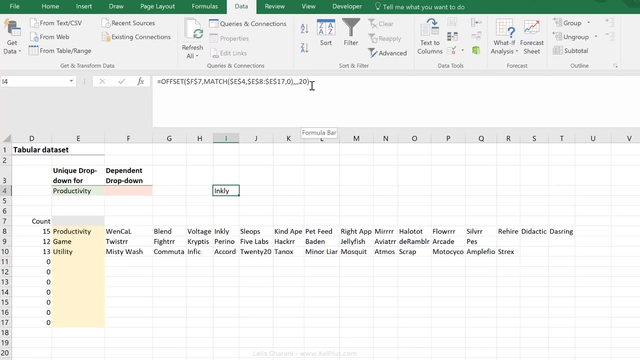 and just put 20 in there. Okay, so if I click on this and press F9, I can see the list and I see the empty ones. So control Z to go back. But the better approach is to also restrict this. Now the formula that I came up with to restrict this. 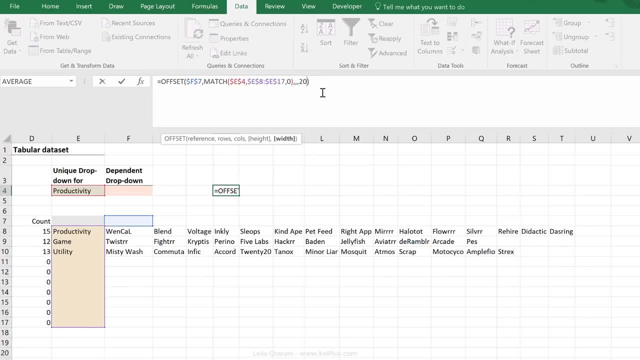 is a combination of COUNTIF and offset And, since this video is already getting too long, I'm not going to explain this in this video, but I'll create a second video on just this concept: how you can restrict your data validation lists to the number of categories that you have. 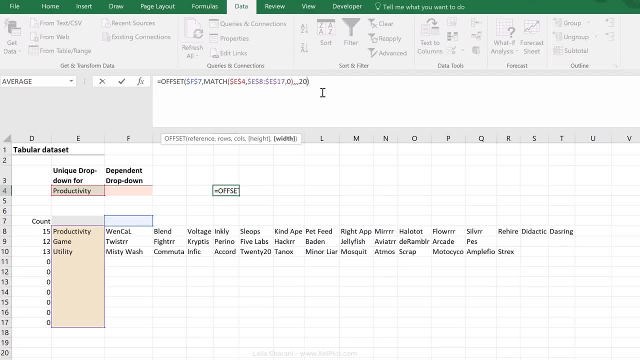 in a separate video And I'll try to get that out in the next month or so. Okay, for now I'm just going to paste the formula in. That's the formula. If I click here and press F9, we can see that now it's restricted to our list. 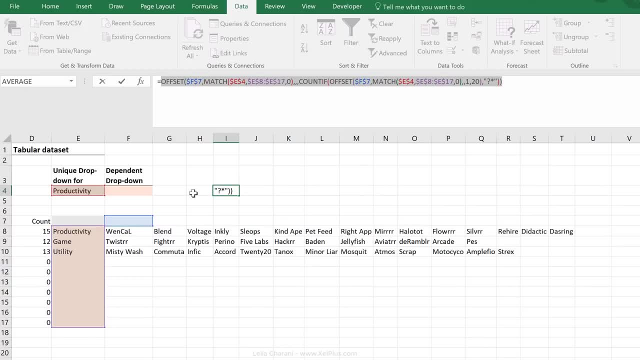 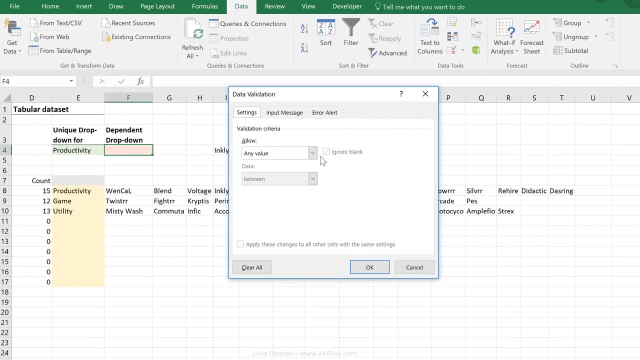 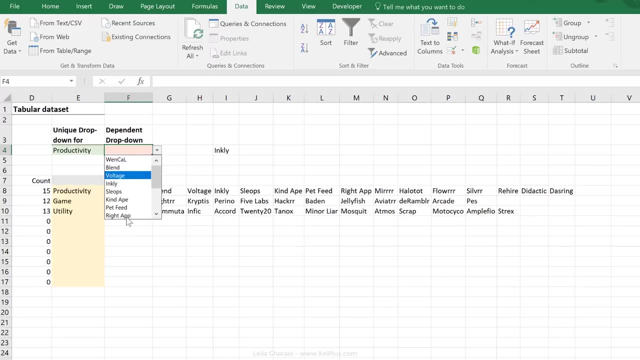 Let's fully test this by copying this and pasting it in the data. So let's go back to our validation box. Go to data data validation, click on list and paste this in. Now let's just double check Venkal blend.